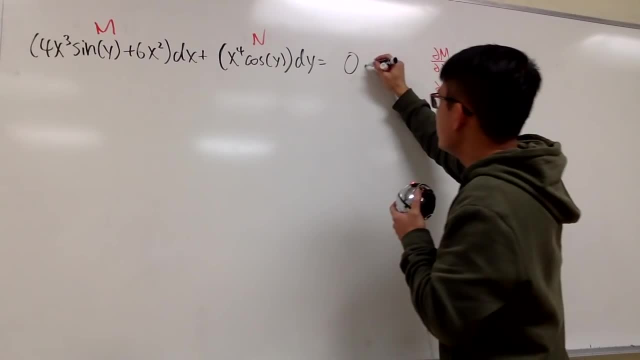 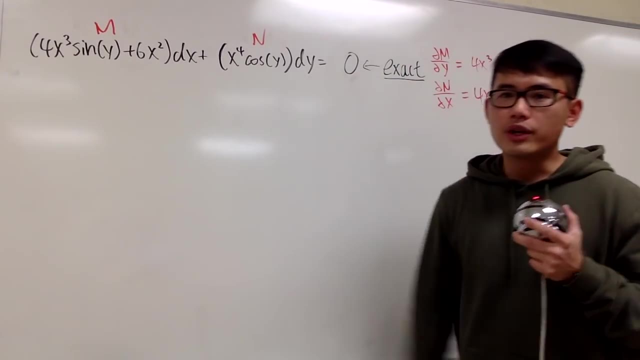 see, these two are the same, So that means this right here is exact. Okay, All right, So we have an exact equation. Everything's nice because we know how to solve an exact equation already. right? You can watch my other video for that. 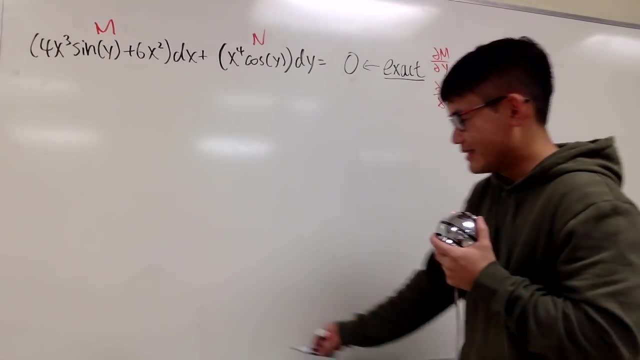 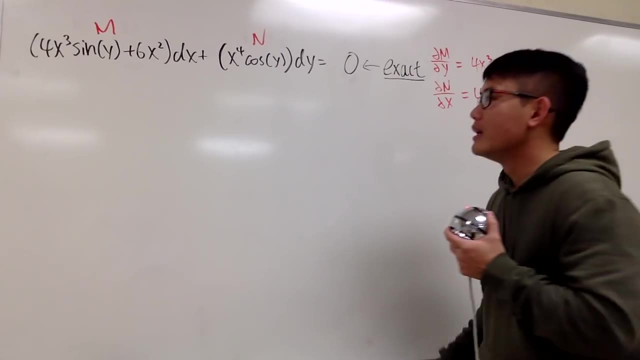 Um, but this is what happened. As I was mentioning earlier, somebody you know takes out this blue marker, and this is what he is going to do. So he takes a look at this exact differential equation and he's not so happy about it because this is so perfect, right? 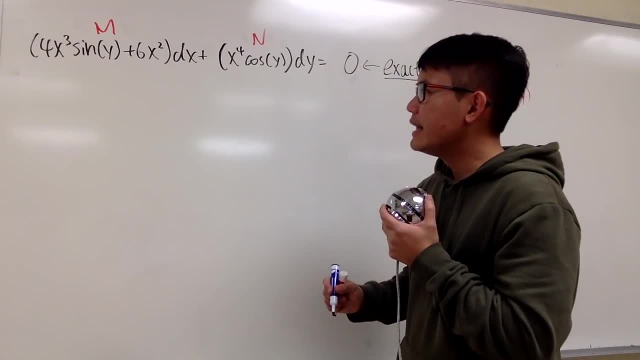 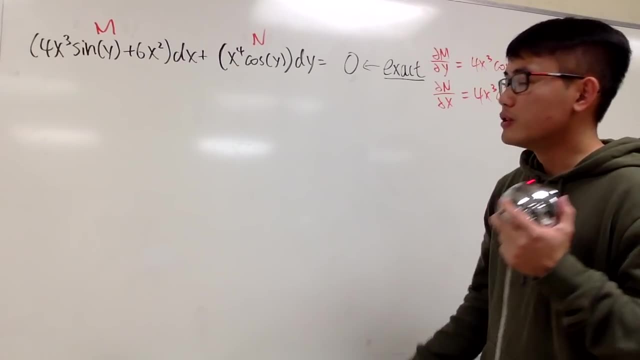 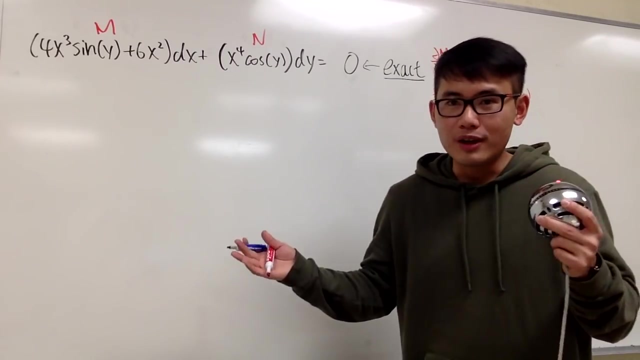 Well, as I said, he takes out this blue marker and he sees that, well, it seems like we have a lot of x to a power in these terms. So what he's going to do is he's going to divide out everything by x to the third power. Well, he can do anything that he wants, but let me just say 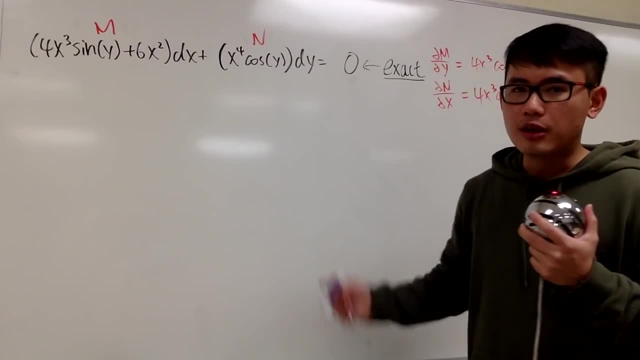 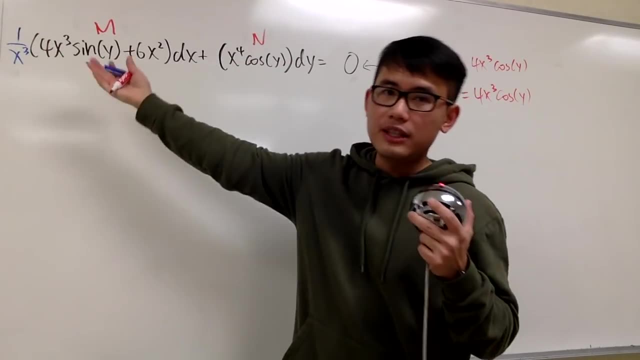 he is going to divide everything by x to the third power, And let me just put it down this way for you guys. Let me write it down as 1 over x to the third power, right? It's the same as dividing everything by x to the third power, right? And let me just write it down here as well. 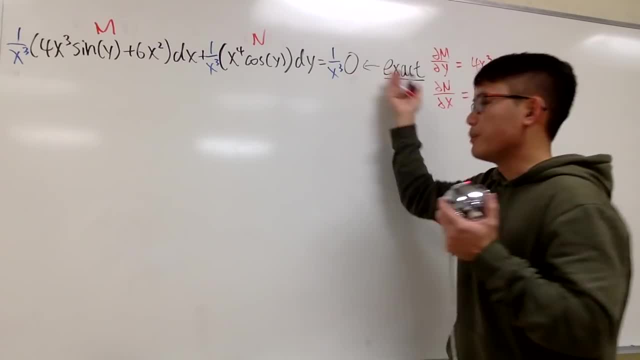 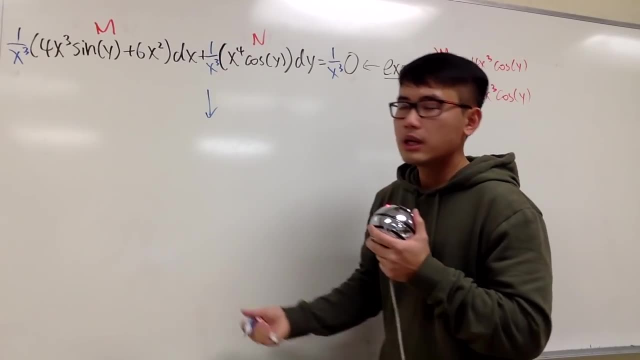 And of course we should also do it on the right-hand side, but that would be 0 anyways. So this is what he's going to do, and then he's going to divide everything by x to the third power. We get another equation, of course, This and that together you see the x to the third power. 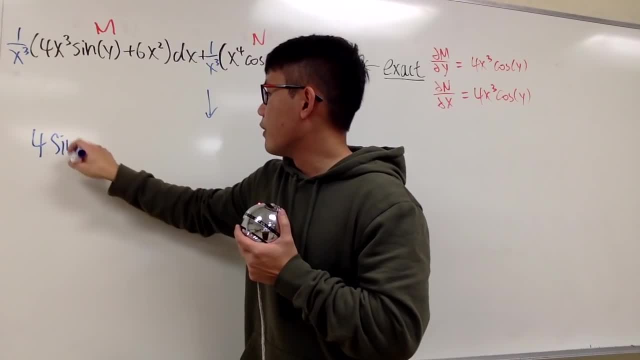 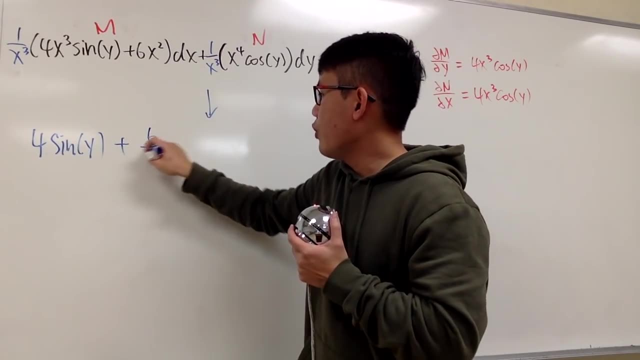 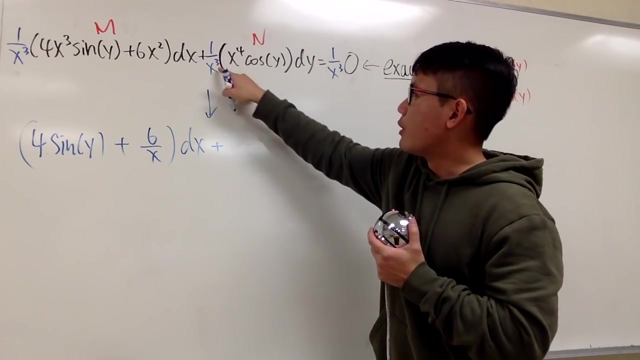 cancel out. so we will end up with 4 sine of y and then this and that we will get plus. we will have x in the denominator right, So we have 6 over x and then close the parentheses and we have the dx right here And we add it with x to the fourth power over x to the third power. 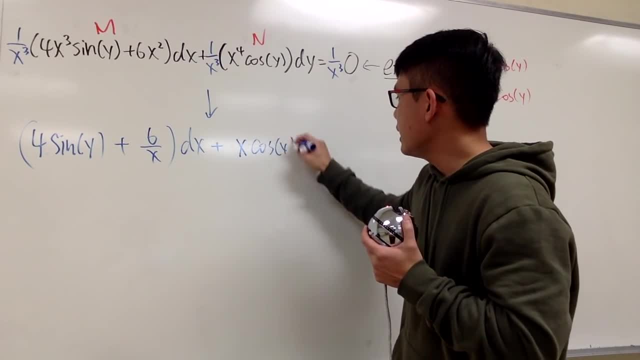 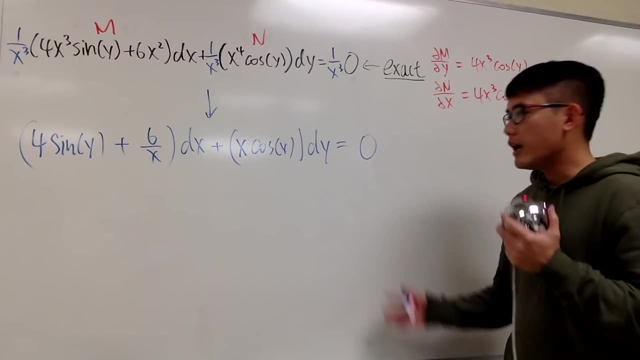 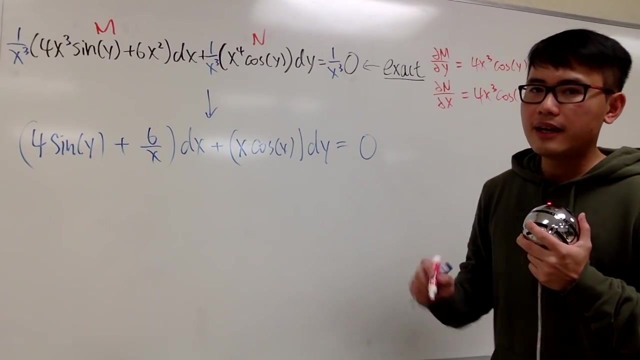 it's just a regular x, and we have the cosine of y, and this is with the y and this and that, of course, it is still 0.. Okay, so now we have a different differential equation, and this is unfortunately not an exact equation anymore, and let's do a real quick check. 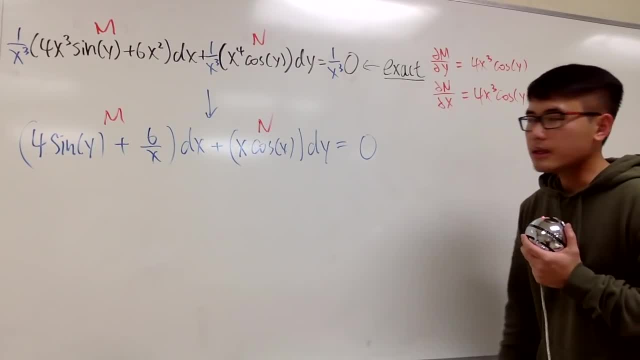 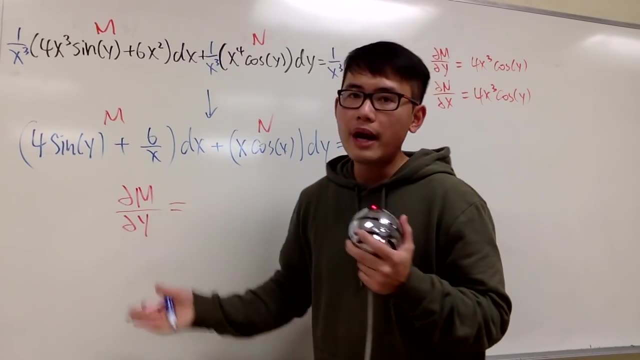 This is m, this is n. okay. So right here, let me just put it down here for you guys. We take the partial of m with respect to y. y is the variable. we only care about this. pretty much right. The. derivative of 4 sine y is just the derivative of 4 sine y. So we take the partial of m with respect to y and we only care about this. pretty much right. The derivative of 4 sine y is just the derivative of 4 sine y. 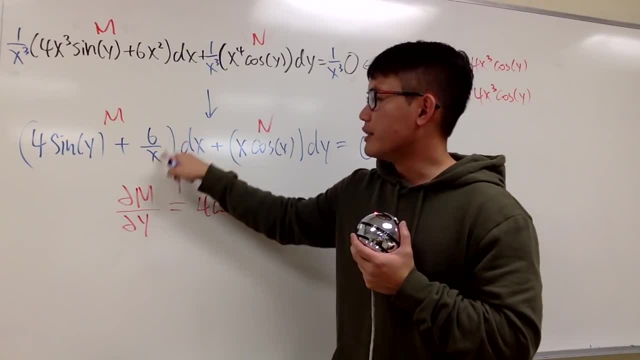 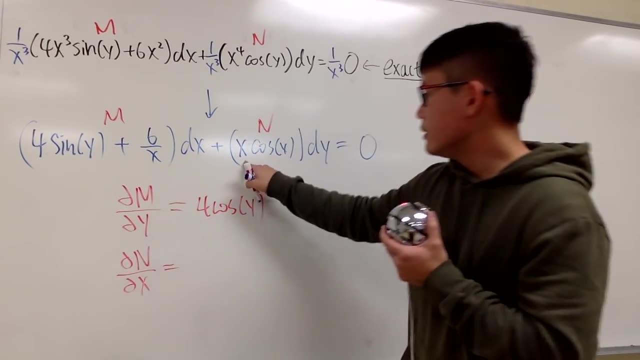 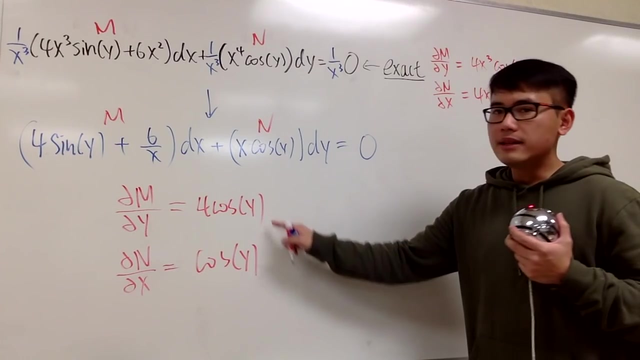 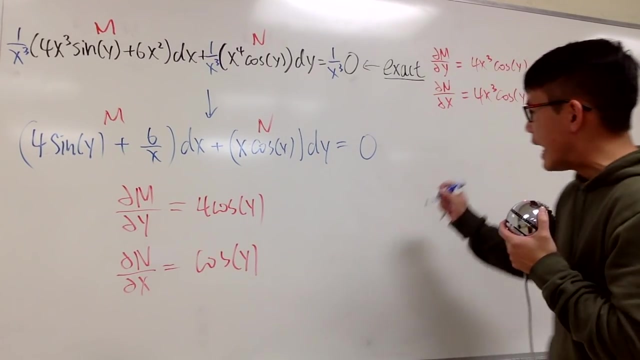 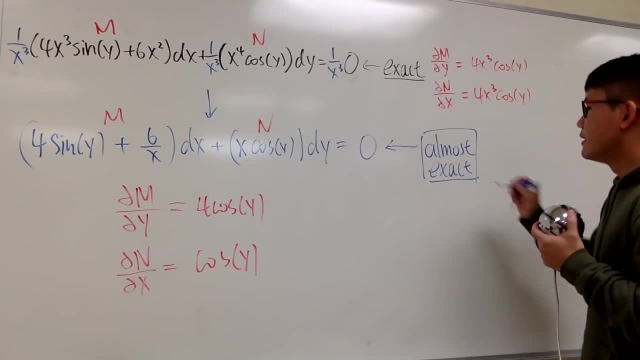 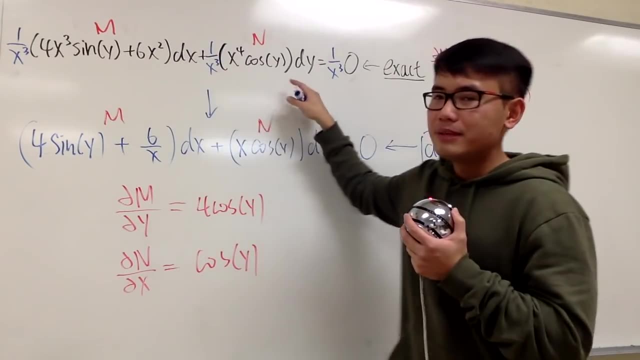 Okay, And the deal is that, because this came from an exact differential equation and you know, the only thing that the person did was he multiplied everything by 1 over x to the third power, Or he divided everything by x to the third power. Same thing, right. 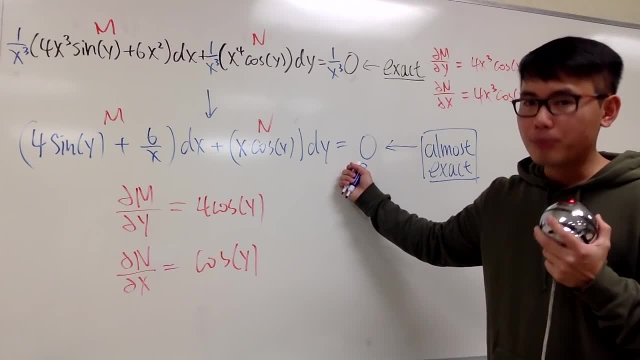 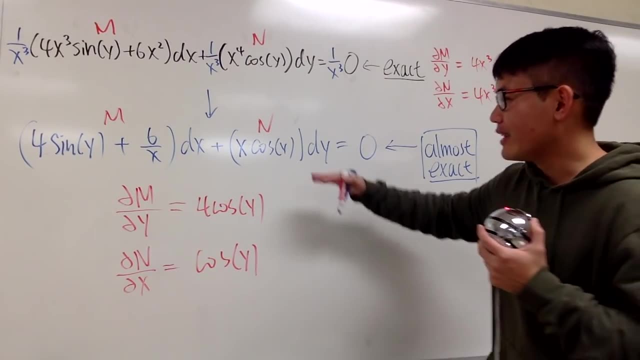 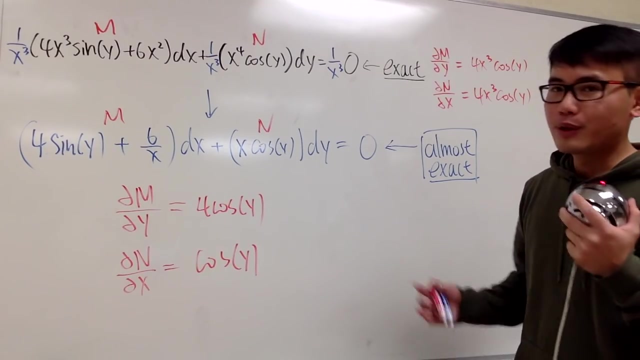 Well, this is in fact not a bad problem at all, Because as long as we can figure out what did the person do, we can just undo it so that we can go from this back to the exact differential equation. everything will be perfect again, right? so here is the question. if this is the 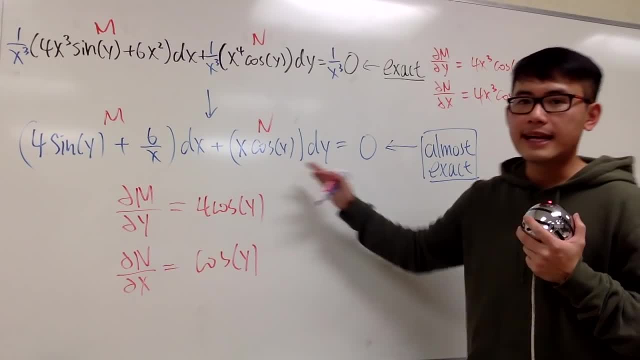 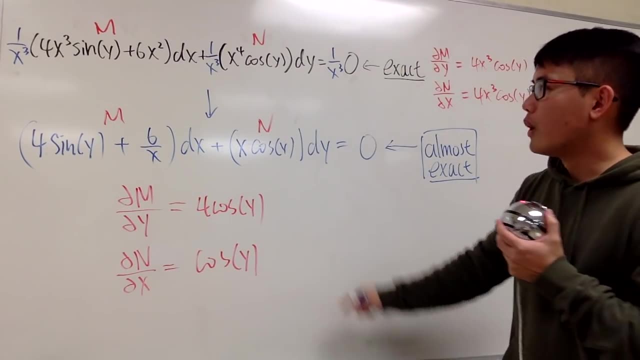 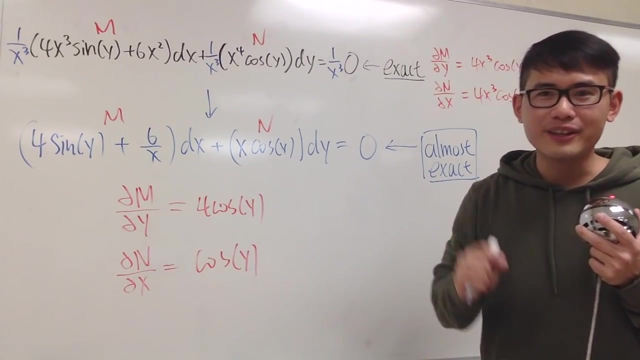 differential equation that we want to solve. you'd know this is not exact, right? how can we make this into an exact equation? how can we figure out what did the person do to us? so let's take a look of what we call the special integrating factor right now. so here's the idea. assume this is not exact at the moment. 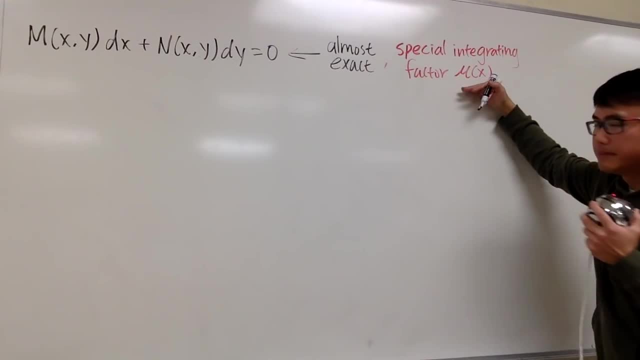 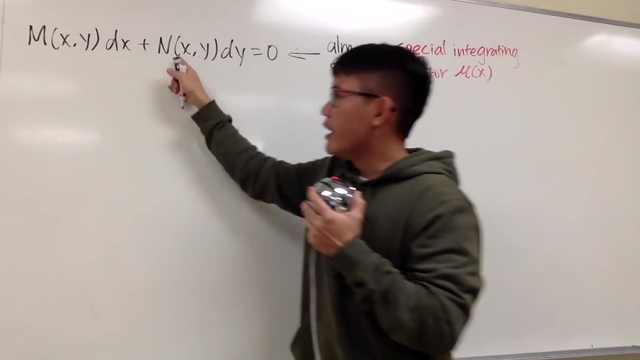 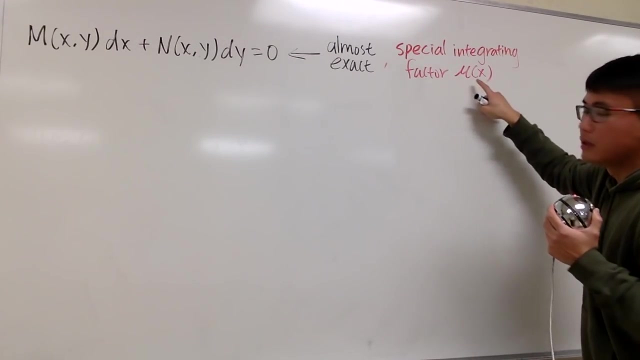 however, after we multiply everything by this special integrating factor, the result of that will be exact okay, and you know the m and n. they are both functions of x and y. however, let's first come up with a formula for the special integrating factor in terms of just X. so we'll call that mu of X and later. 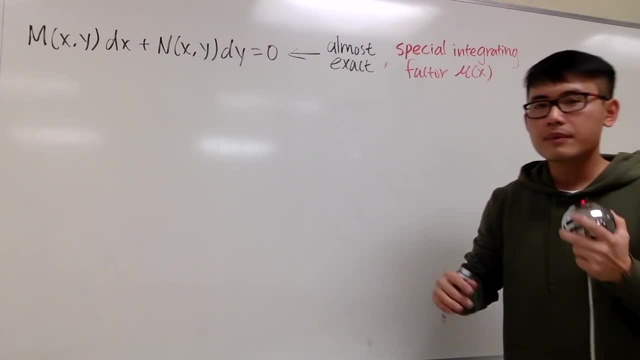 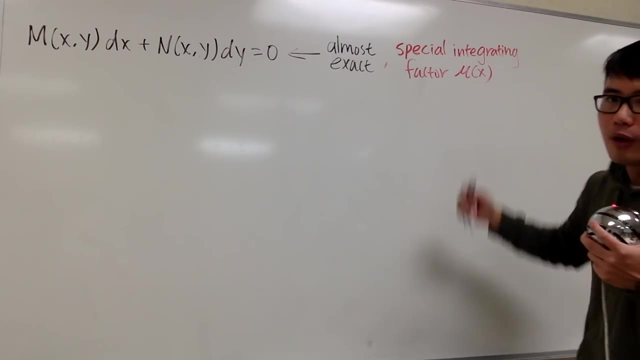 on. also show you a formula for mu of y, a special integrating factor in terms of just y and, of course, the special integrating factor in terms of y. and of course the special integrating factor could be both a function of x and y. But seriously, we hope that doesn't happen. 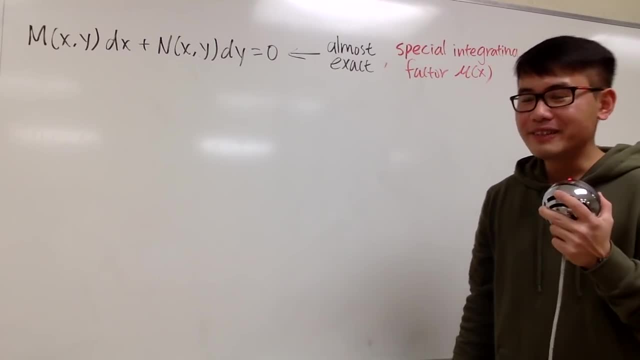 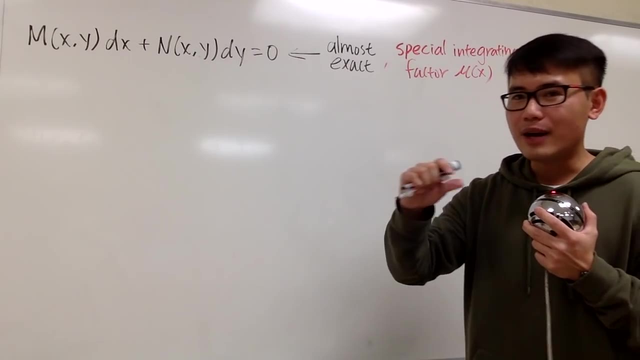 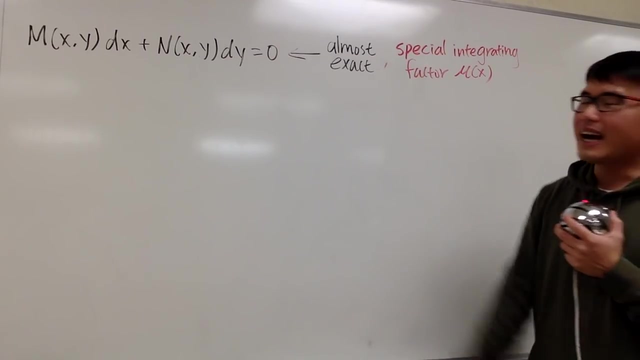 because the computational part is going to be really hard. So, hopefully, this almost exact equation. it came from an exact equation that somebody just defined out, either just in terms of x, or an expression in terms of just y, and things like that. Anyways, let's get started on. 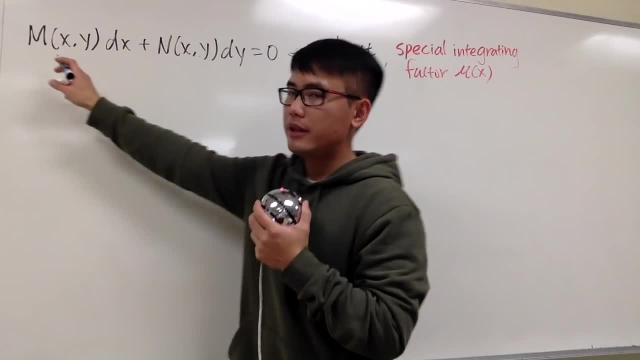 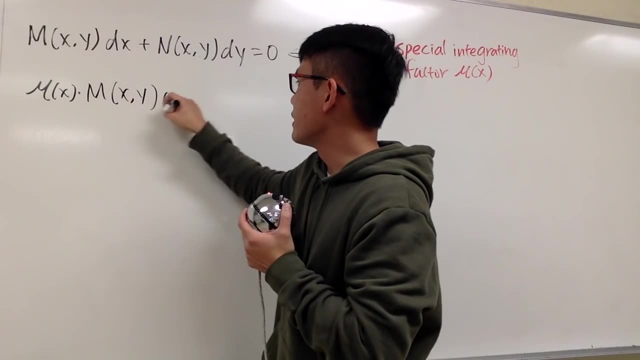 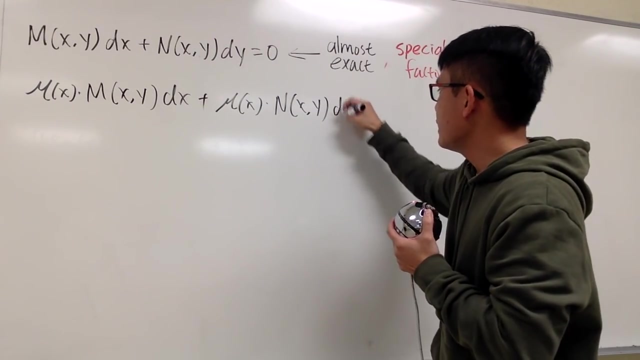 that Let's multiply everything by mu of x. So let me put it down right here for you guys. We will have mu of x times m of xy and we have the dx and we add it with mu of x times n of xy, dy and. 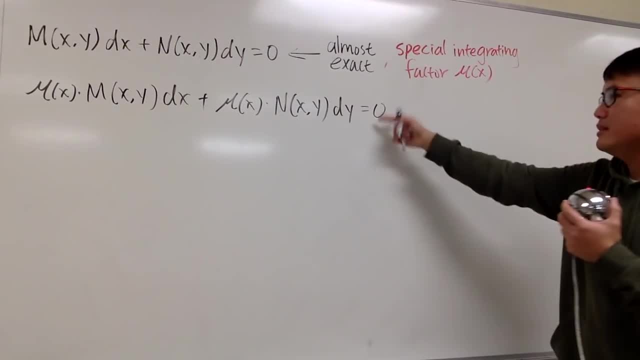 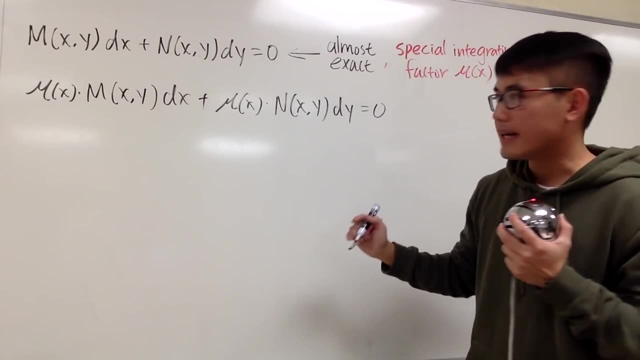 this is still equal to zero, because zero times that is still zero, right, All right, this right here. it was not exact. I call that almost exact, But after we have the mu of x right here, this right here, we want it to be exact. 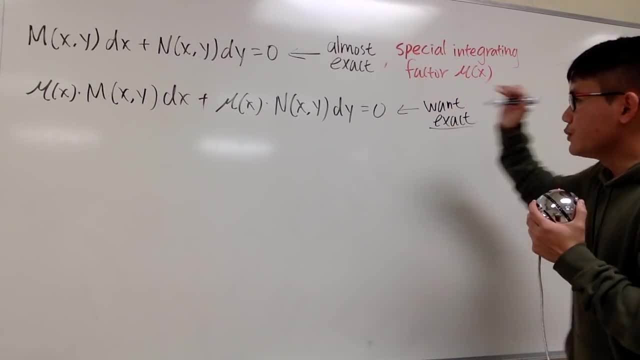 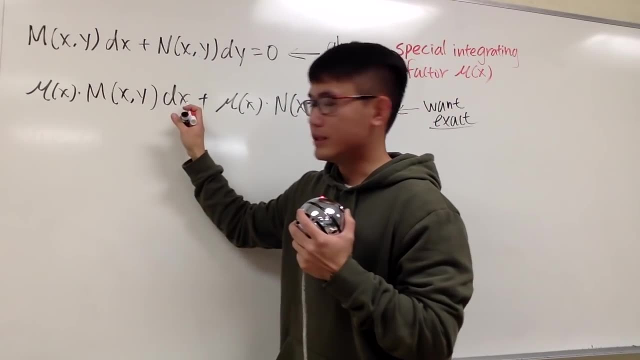 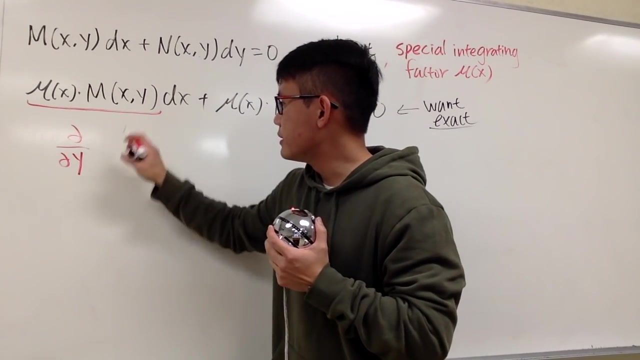 Okay. So once we know this is exact, we know we have to do the mixed partial derivative right. So we'll take this and this is with dx and it's the whole thing right here. okay, We will take the partial with respect to y of this right here. So it will be mu of x times m of xy. 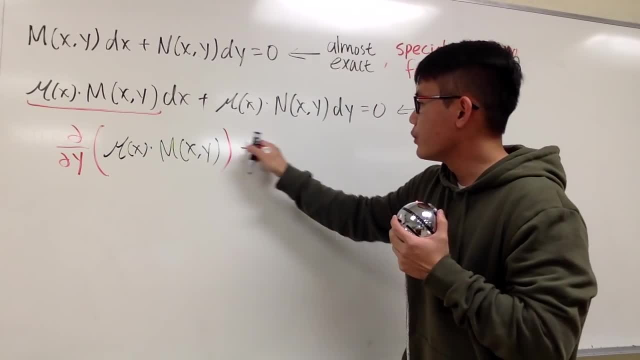 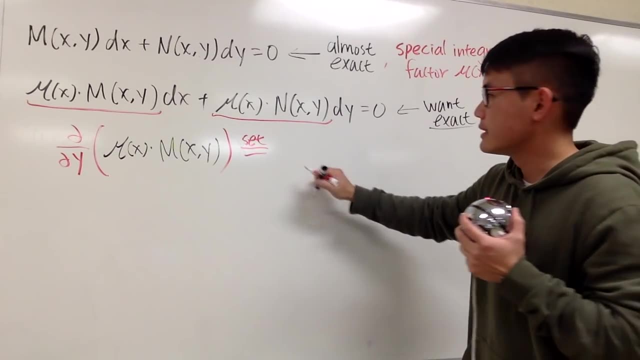 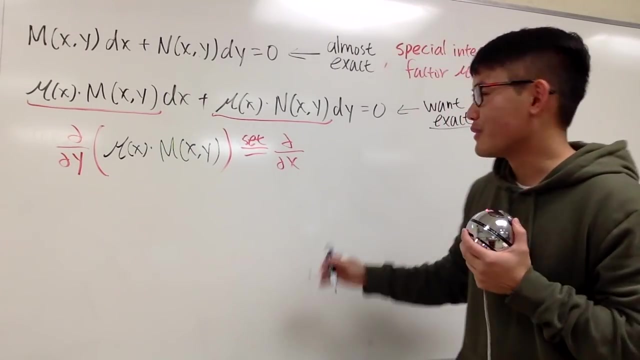 and we are going to make sure we set this equal to. we take the partial of this with respect to x, because we know, if you want this to be exact, the partial derivative, like this, will be the same right. All right, so put this. 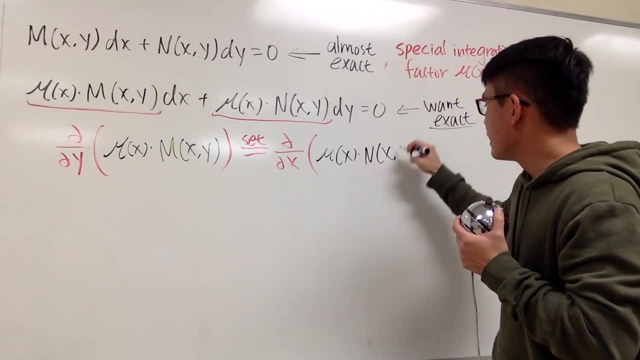 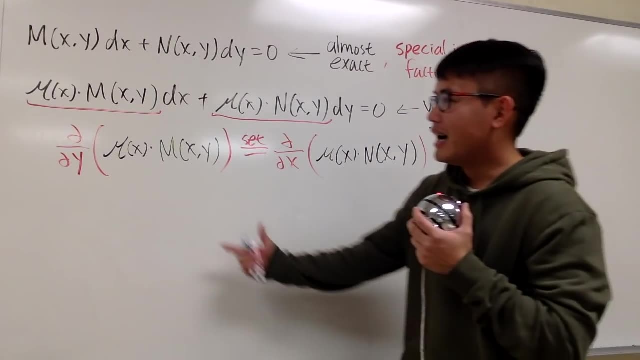 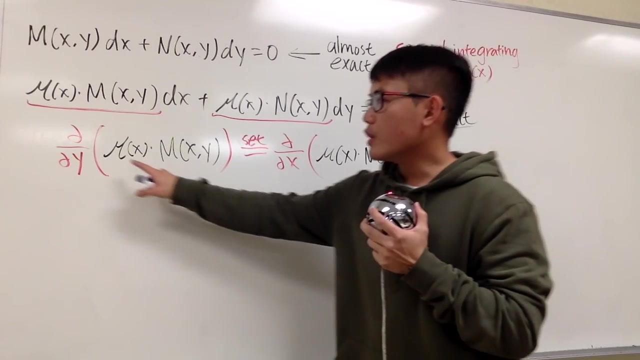 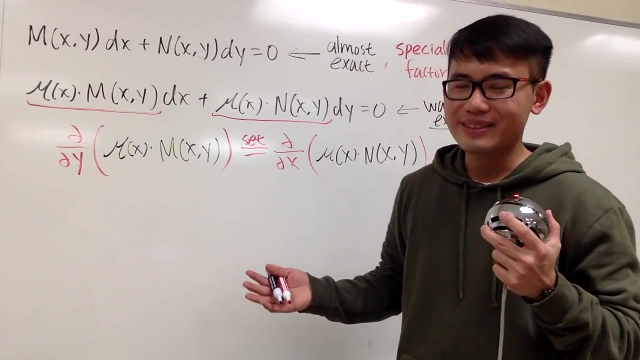 down right here: mu of x times n of xy, like this. And now let's do some partial derivative On the left hand side. yes, it is a product of two functions: mu and m. However, we are doing the partial derivative with respect to y. Mu of x is considered to be a constant. 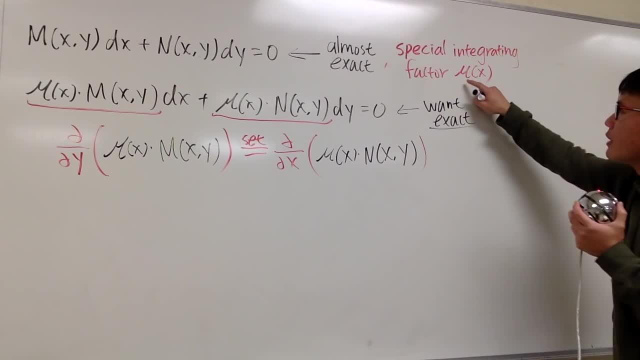 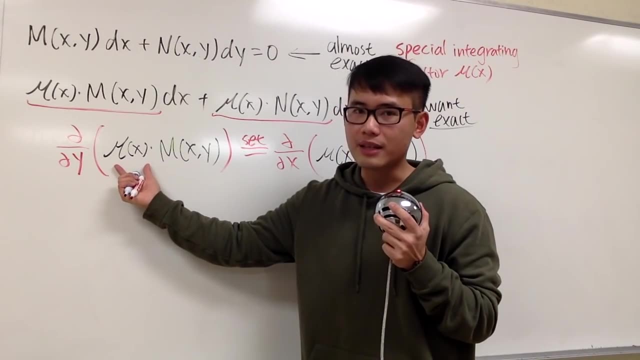 right, And you see, this is the reason why I want to just first talk about mu of x, a special integrating factor in terms of just x first, Because mu of x will be considered a constant in the y world. I don't have to use the product rule right here, So it saves some work, right. 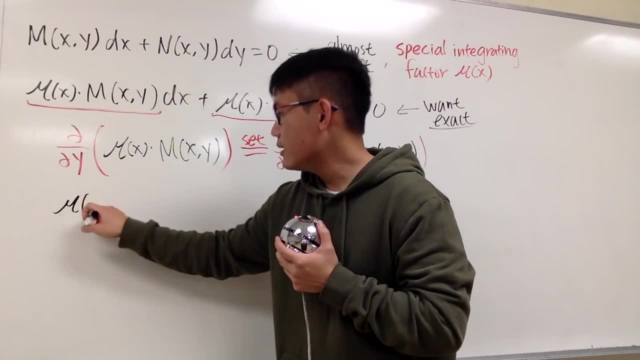 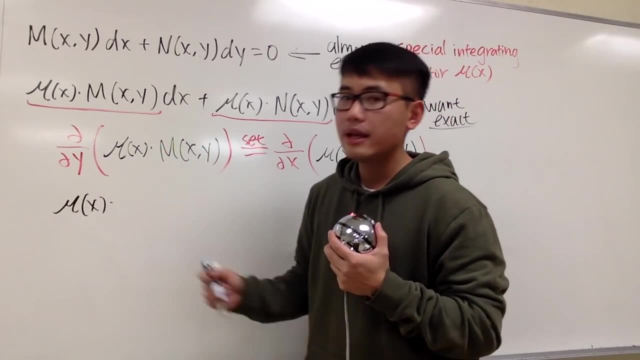 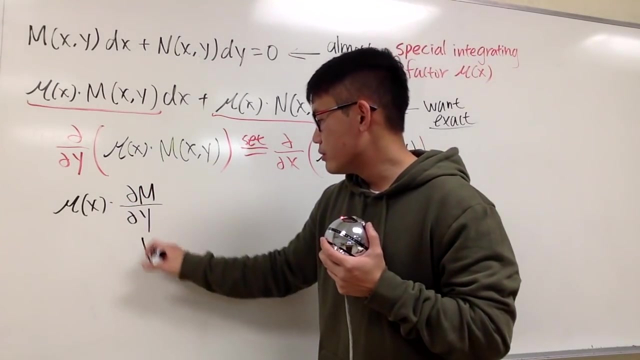 All right, so let me just write down the constant mu of x in the y world And then we multiply by. let's take the derivative of m with respect to y and I'll put this down as partial of m with respect to y like this, And later on I'm going to show you with this: 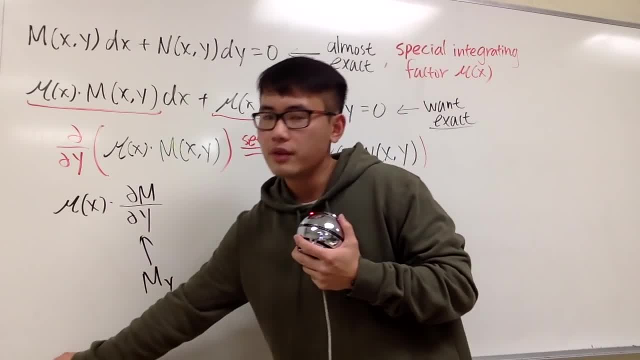 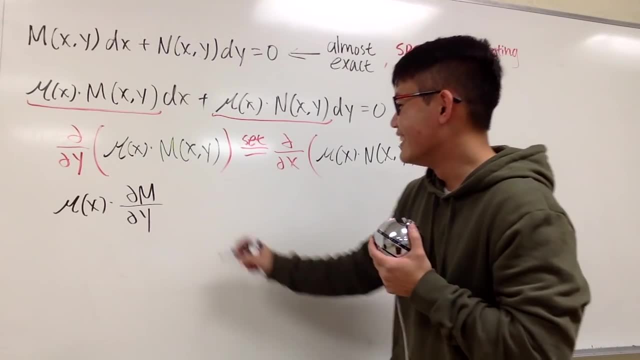 notation m sub y for the partial derivative. but let me just keep this for now. throughout my computation, And this is it right? That's the beauty of this. And you know m is a function in terms of both x and y. but let me just write down m right here, okay, And this is: 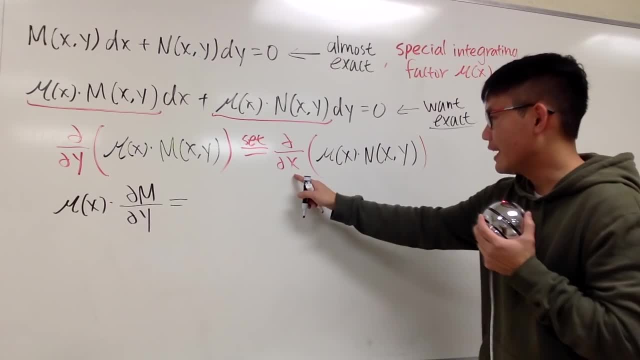 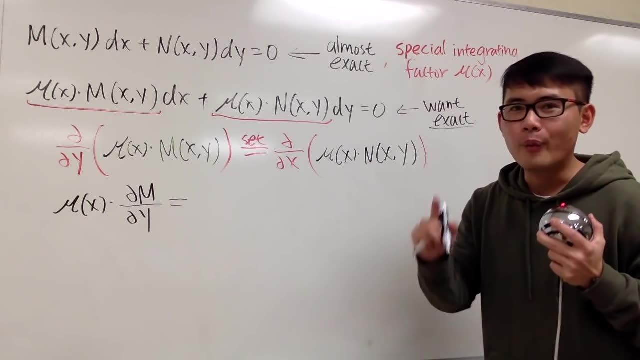 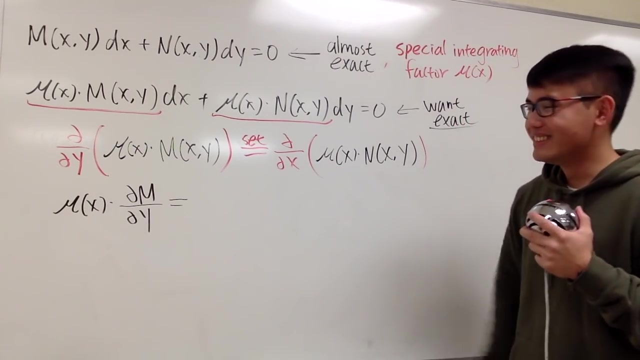 equal to. here we are taking the partial with respect to x of mu of x times n of x. Both of these functions contain x. therefore we have to use the product rule. So we cannot avoid not to use the product rule. okay, We have to do it right here, But it's better. 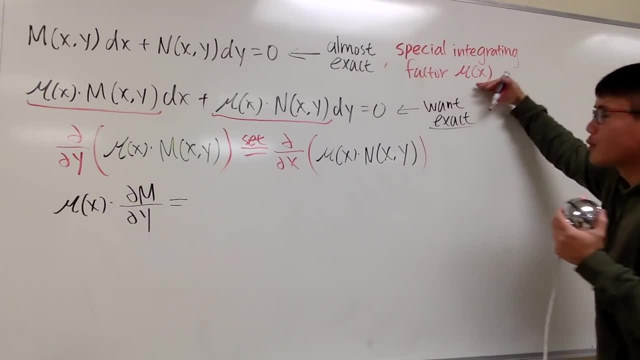 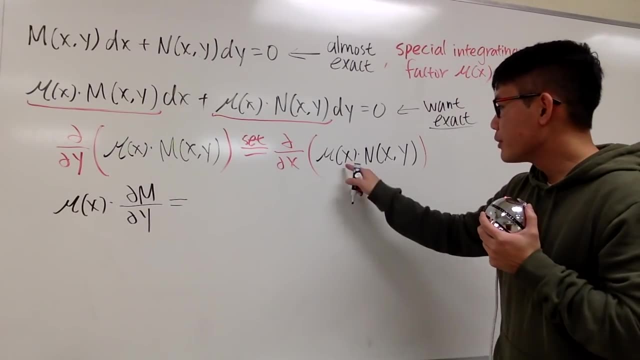 than do the product rule both sides. So, once again, this is the reason why we restrict to the special integrating factor in one variable first. Anyways, here's the product rule. I'm going to keep the first function. This is the first function, which is mu of x, And we multiply by the derivative. second, 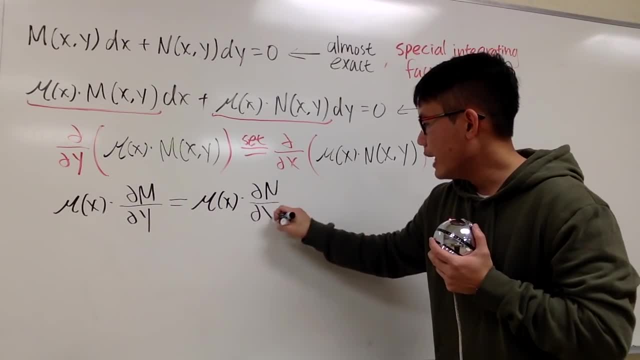 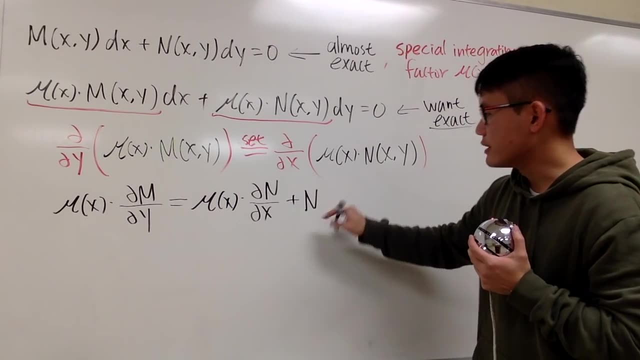 I'll write that down as partial of n with respect to x. Okay, that's the partial derivative with respect to x, And we add it with the second function. I'll just write that down as n. n is the same as n of xy. okay, And we multiply by the derivative. first, I'll 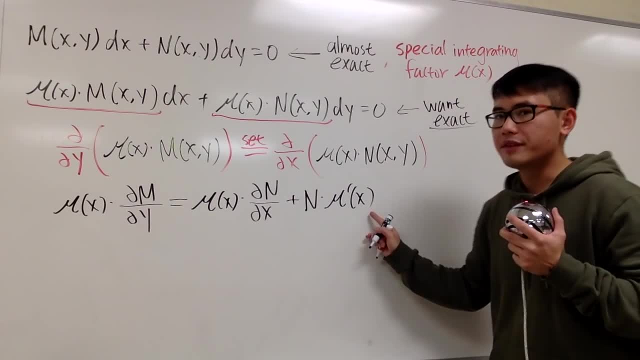 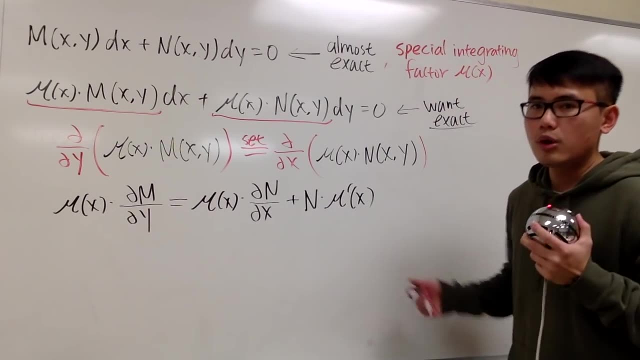 write this down as mu, prime of x, the usual derivative formula in one variable. Okay, so now we are going to see how can we find the derivative of the first function. So let's see how can we find a formula for the mu of x. This is similar to the special integrating. 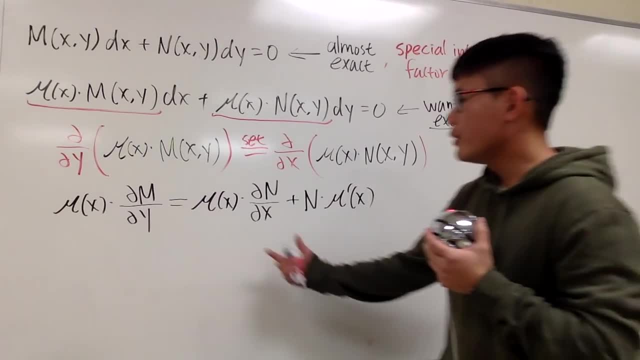 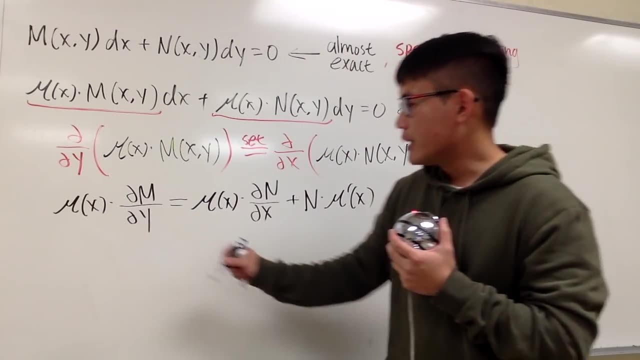 factor for the linear differential equation. So here's the deal. I'm going to move this to left hand side because they both have the mu of x right, So I can also factor that out. So let me factor that out first, mu of x, and open the parenthesis. This is still. 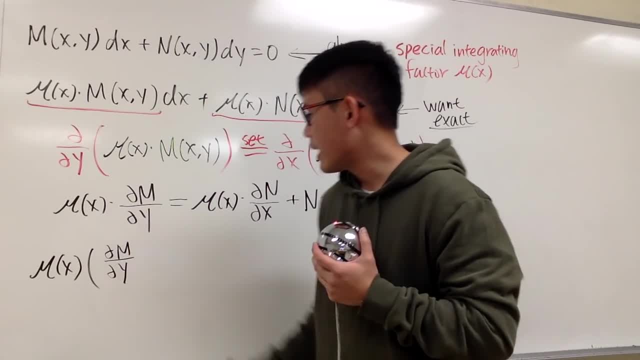 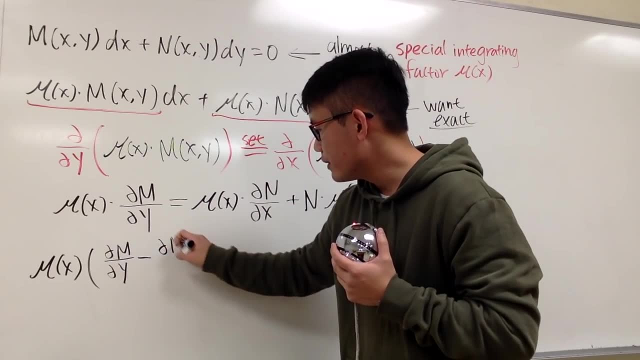 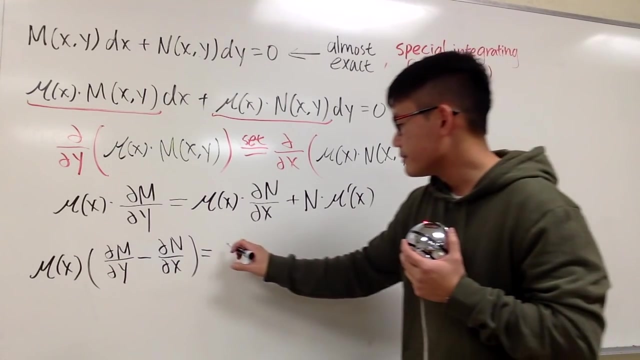 positive. so I'll write that down as partial of m with respect to y And once I move this to left hand side, This will be minus right. So we have the minus part of n with respect to x like that And this is equal to: we have this on the right-hand side: n times mu, prime of x. 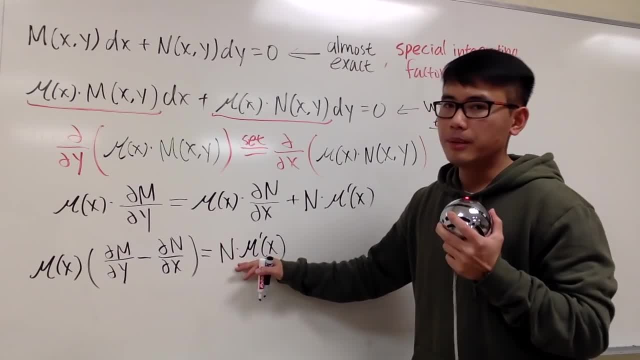 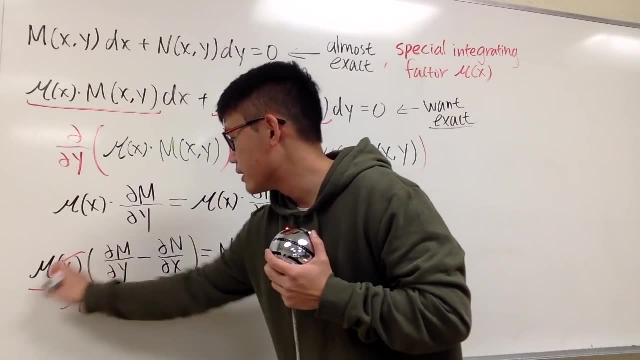 And now, what I'm going to do next is: I would like to keep the mu prime of x on the numerator, so I'm going to divide both sides by the mu of x, And if you have seen such a computation in the past, 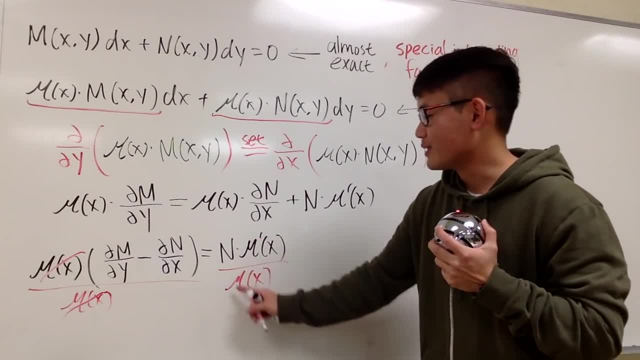 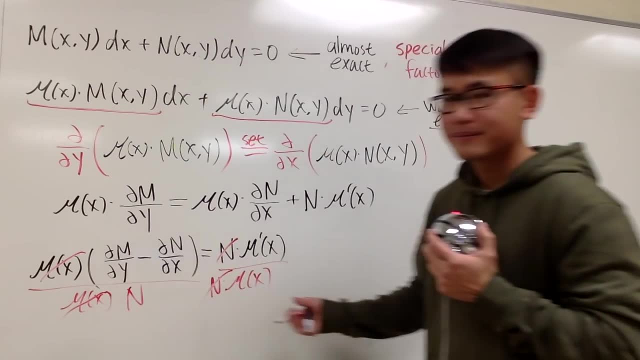 you know this right here is just the derivative of a natural logarithm, right? Anyways, I don't want the n, though, so let's divide both sides by n, like this: Cancel, I can move that to the other side. Alright, so here we go. I'm going to put this down right here. 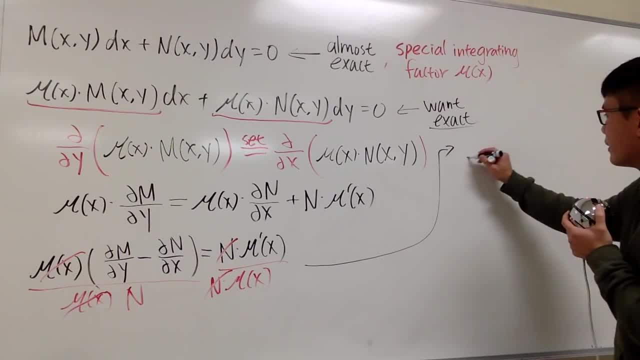 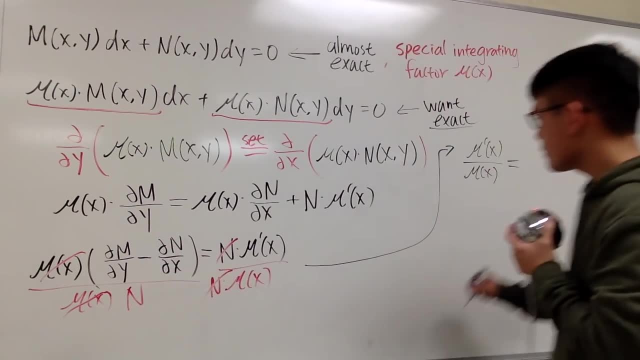 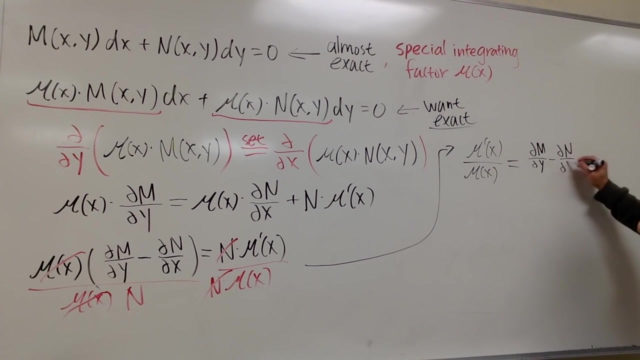 On the left-hand side. let me write this down first. okay, We have mu prime of x over mu of x, and this is equal to this right here. So we have the partial n with respect to y minus partial n with respect to x. 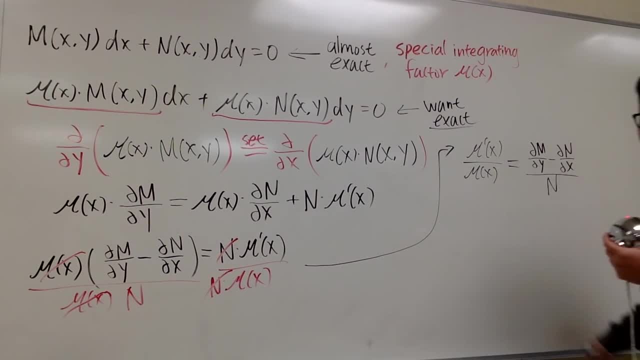 all over capital N, like that. Okay, now here's the deal. We have to integrate this right, Because that's how we can get rid of the derivative. and we will integrate this with respect to x, And we'll do that on both sides, of course. 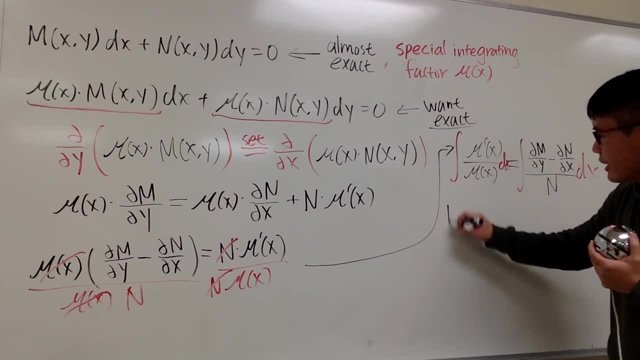 And you know this right. here is nothing but just the natural log absolute value of mu of x. Well, how do we know? Because if you write this down, you take the derivative of this. you put mu of x on the bottom. 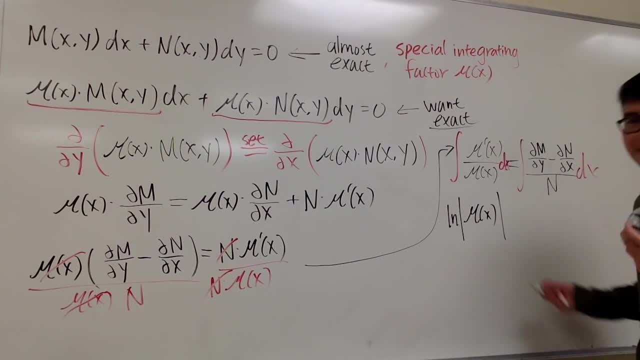 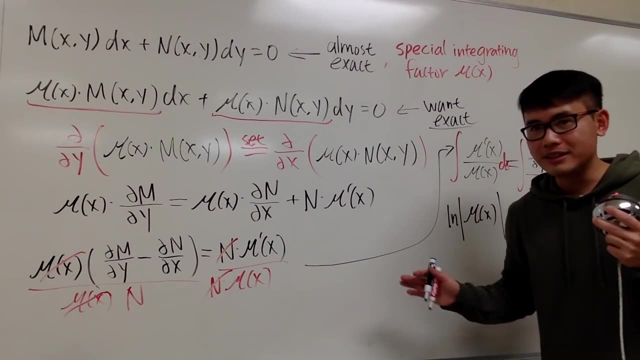 and because of chain rule, you put the derivative of mu on the top right. So this is the beauty: we can just integrate that and get this. And for integrating factors, you don't need to worry about the plus z on the left-hand side or on the right-hand side. 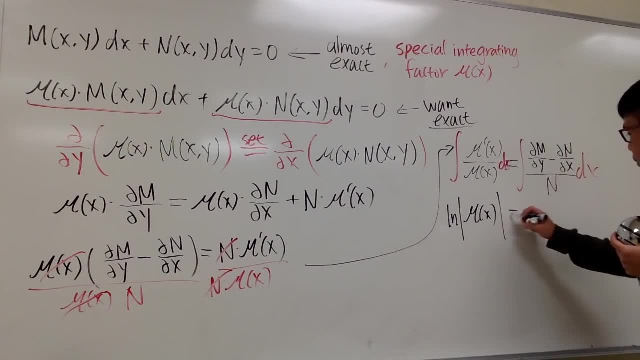 Just, you don't need a plus z at all. Okay, this is equal to that. uh, it's the integral partial m with respect to y, minus partial n with respect to x, all over n, and we have this dx right here. 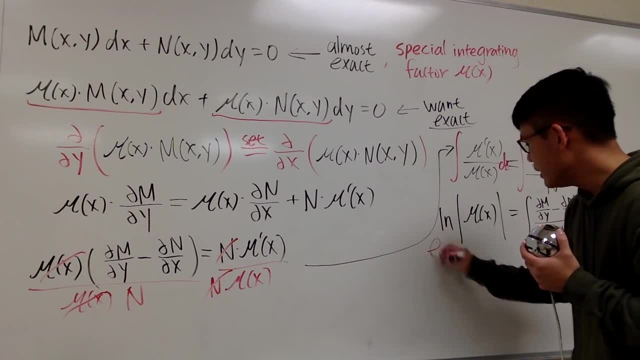 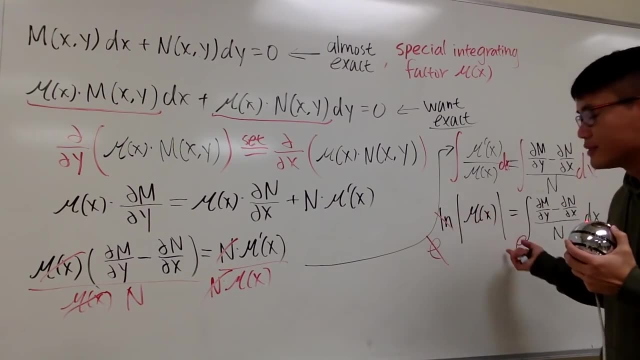 Okay, of course we want to get rid of the natural log. so let's do e to this power and let's do e to that power, so that this and that will cancel On the left-hand side. yes, we should still keep the absolute value, right? 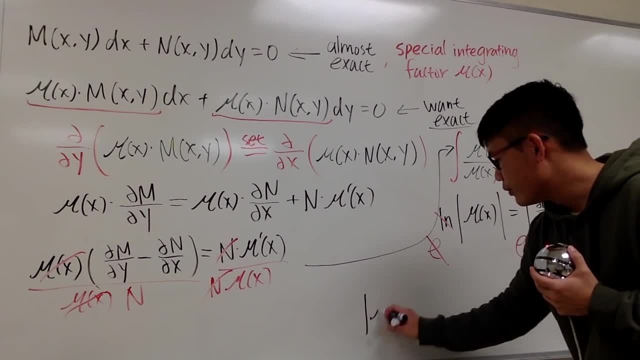 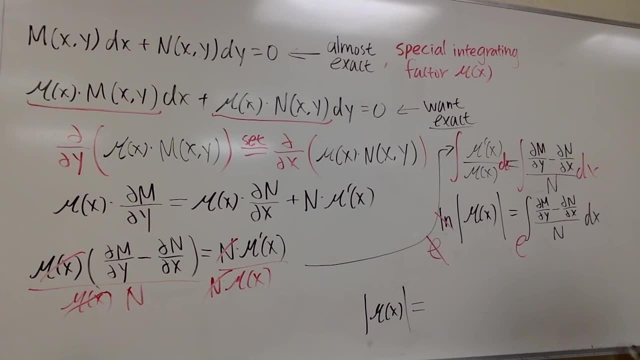 And I will keep this absolute value for you guys. So I will write down absolute value of mu of x and this is equal to: we have this giant expression, We have this expression right here: E is the base and we have this integral as the power. 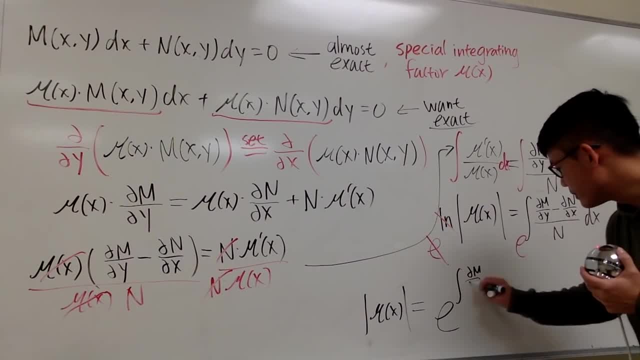 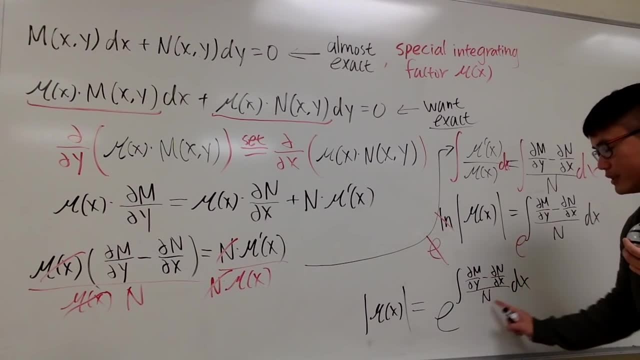 so it's the integral power. We have the partial m with respect to y, minus partial n with respect to x, all over capital N, dx, And notice that everything right here is in the integral. so you have to work this out first and then do the integral. 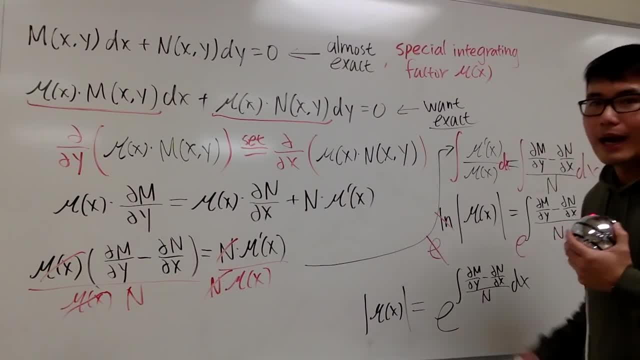 Anyways, we have absolute value of mu is equal to this. How can I get rid of the absolute value? Technically, I can just get rid of the absolute value, but you have to make sure you put a plus- minus on the right-hand side, isn't it? 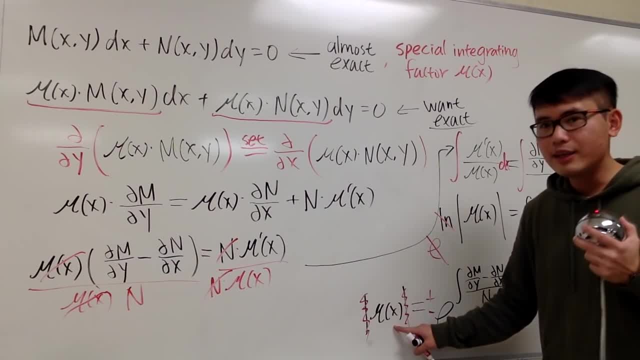 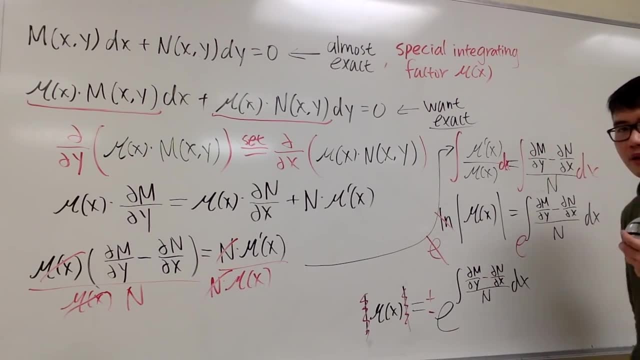 And the idea is that when you want to find an integrating factor, you just need to have one. Right here we're saying: mu is equal to the positive version of this expression or the negative version of this. Which one would you rather use? 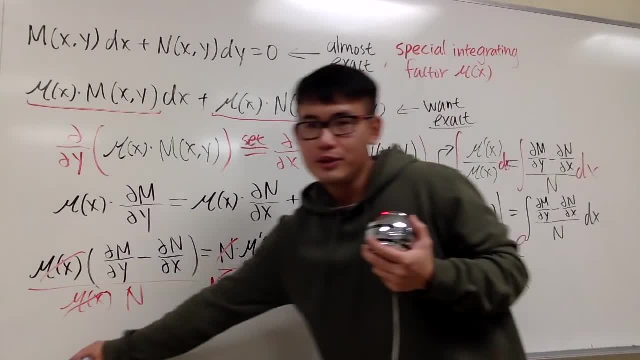 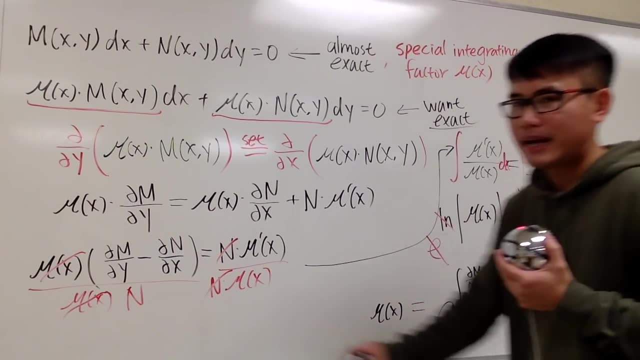 You can use either one right, So it doesn't really matter, And you can just, of course, seriously forget about the absolute value, and even you forget about the plus minus. Let me just say, let's use This right here. 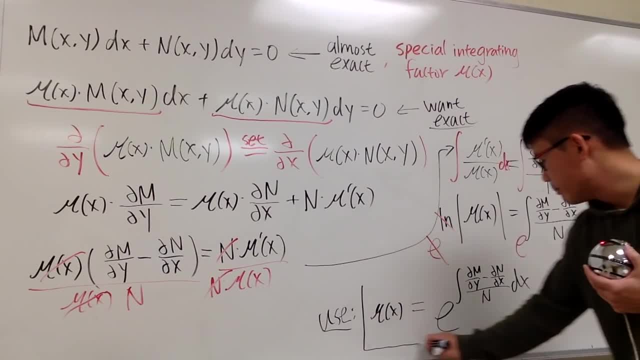 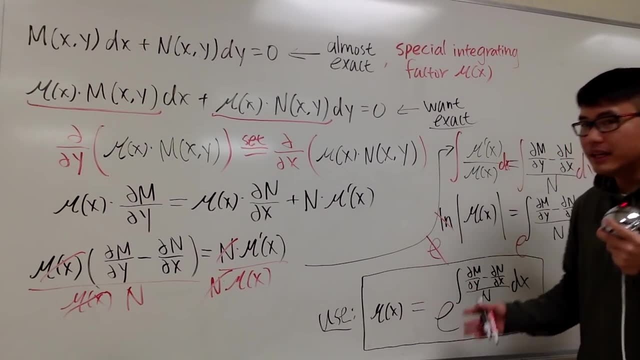 Let's use this formula for the mu of x, okay, So let me box this for you guys. So here we have it. This is the formula for mu of x And similarly we can work out the similar steps. We can work out the formula for mu of y. 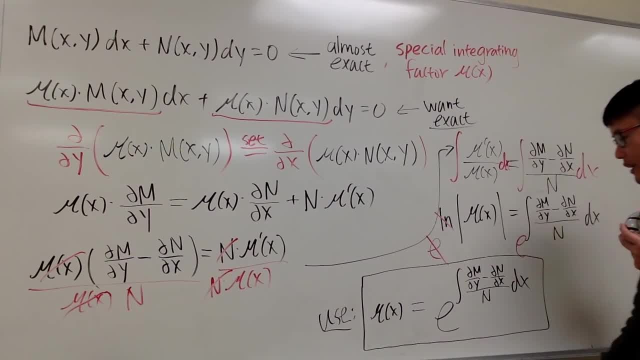 And before I show you guys how to work this out, what was in the example that I did earlier, I want to say that, once you work this out, okay, the partial of m with respect to y, minus partial of n with respect to x or over n. 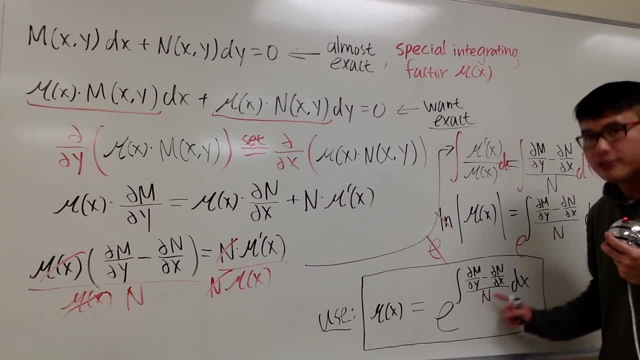 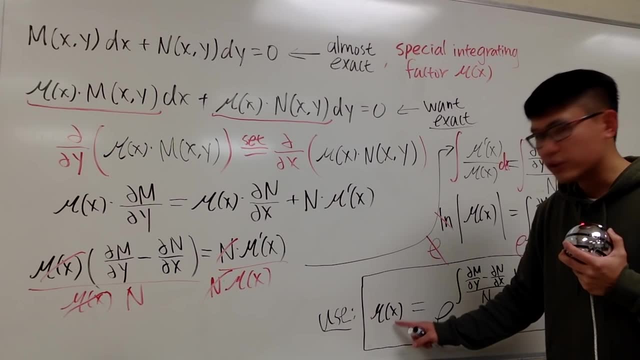 everything right here should contain just x. Y is not allowed at all, Because on the left-hand side you can see, mu is just a function in terms of x. There's no y is allowed right. So we cannot have any y's right here, neither. 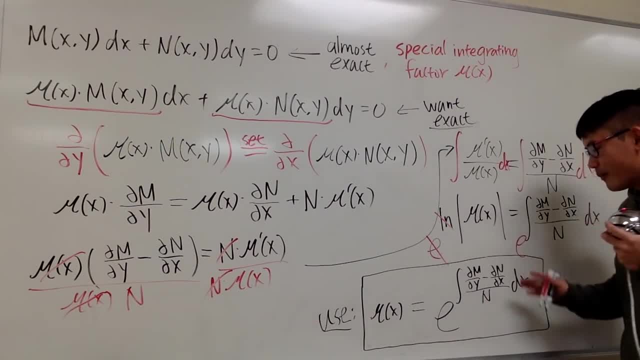 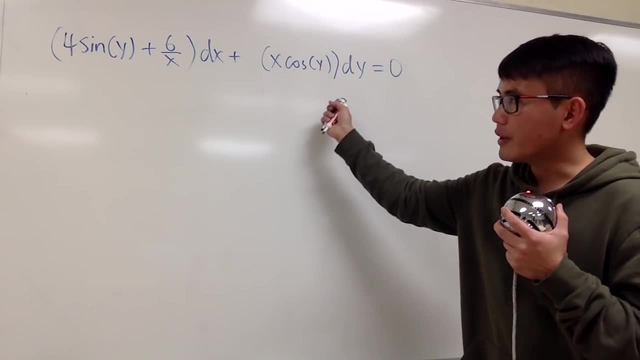 Otherwise, both sides, they will have disagreements. So this is the formula, And now I'll show you guys how to fix the problem that we had earlier. So now let's solve this differential equation And, as we saw earlier, this is not exact yet. 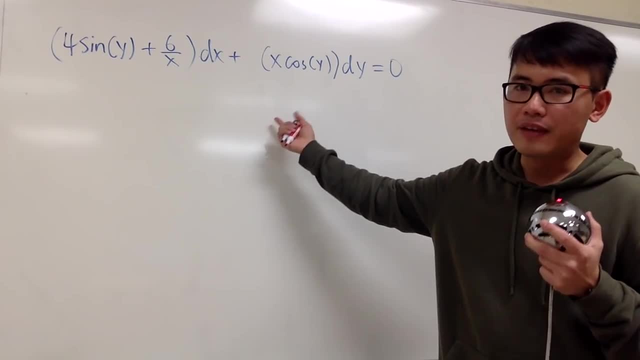 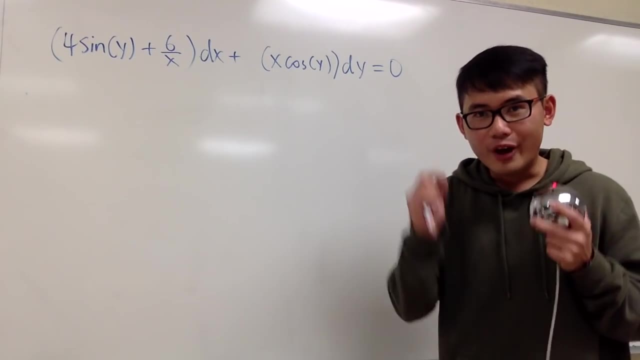 And the usual procedure for exact equation you know does not apply for this at the moment. And here's the thought process: Whenever we're trying to solve an equation that you know it's not exact, we hope that we can find a special integrating factor. 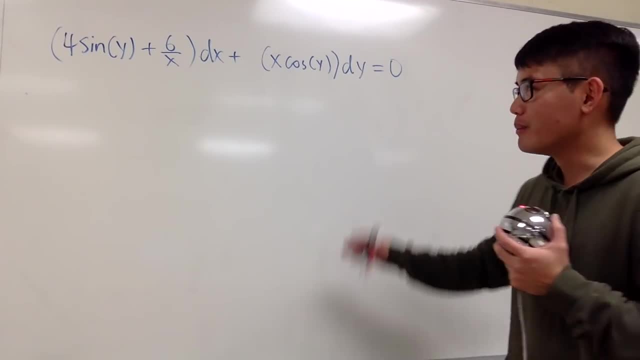 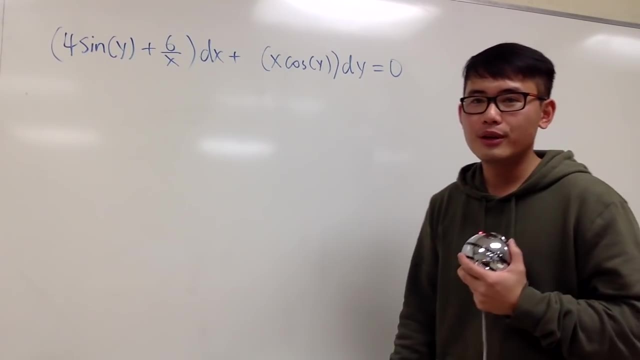 in terms of just x or in terms of just y, so that we can multiply everything by that special integrating factor and the result of that becomes exact, and then we can go through the usual procedure. Well, this kind of equations are hard, okay. 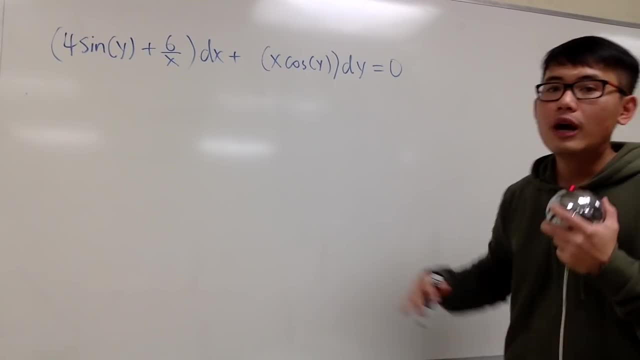 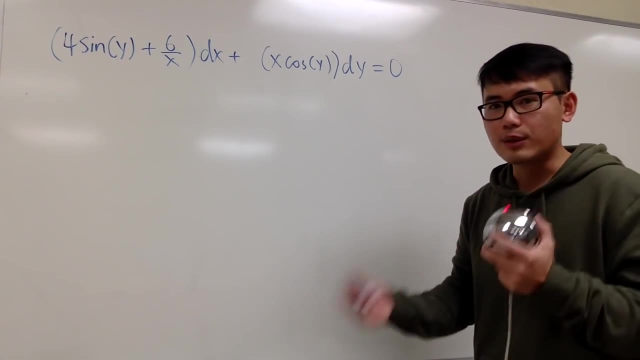 Because if you just give this to us, okay, we can solve it. But if you just give this to me on the test or something, I wouldn't know, do I have mu of x, or do I have mu of y, or maybe mu in terms of both x and y? 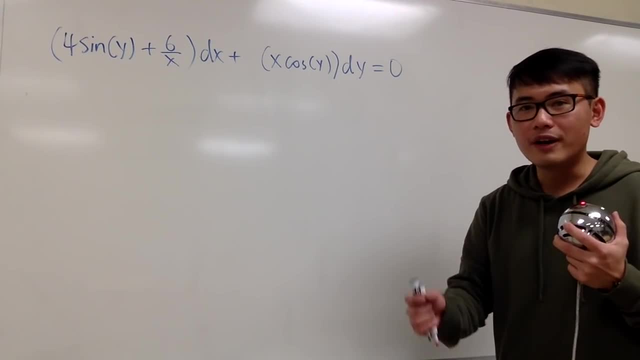 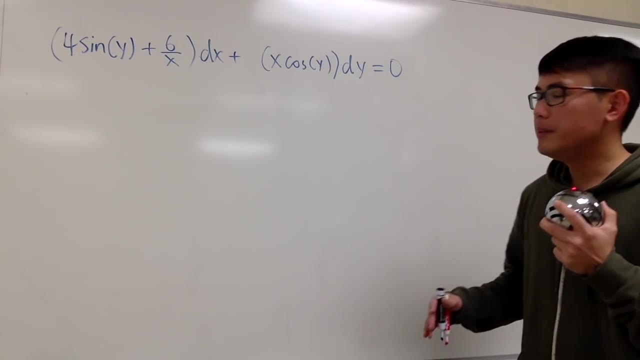 So in this video the purpose is just to demonstrate mu of x. the formula we saw earlier works And then later on you can see in other videos. I'll show you guys how we can think through about it. Maybe I will have a chance to show you guys. 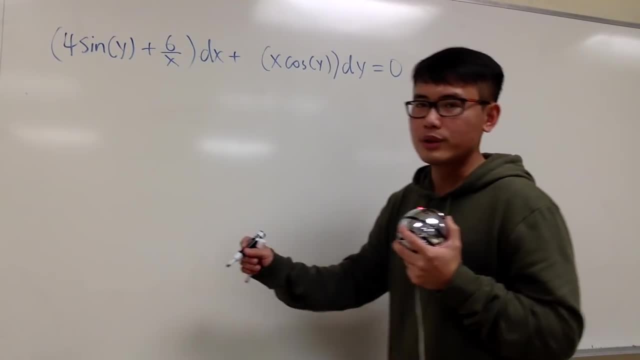 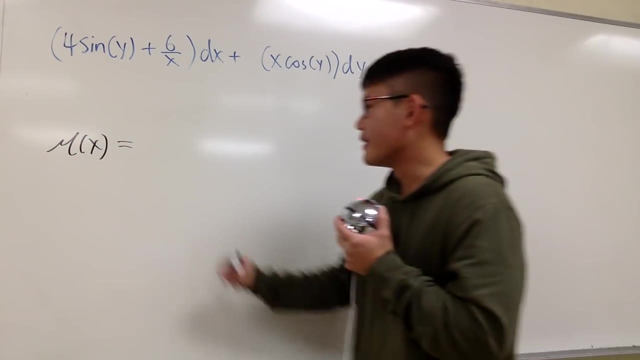 some special, special, special cases as well. But anyways, let's get going with mu of x right here. Let's figure out what do we need. Okay, suppose you didn't see the first part of the video right here. Anyways, mu of x is equal to e as the base. 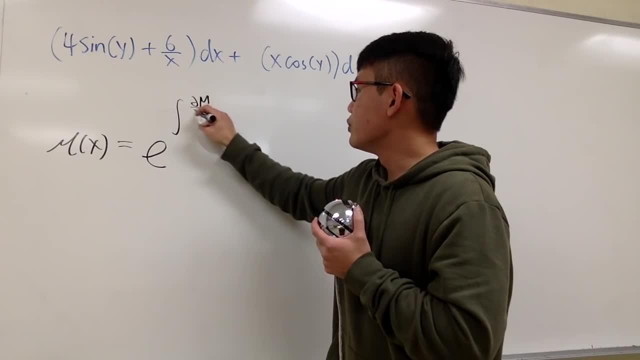 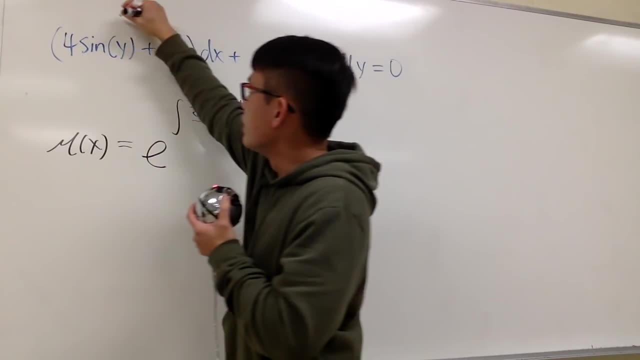 and we have an integral for the power, and it is partial m with respect to y minus partial n with respect to x, all over n, dx, And you know this right. here is the m, this is the n, And hopefully this all becomes just an expression. 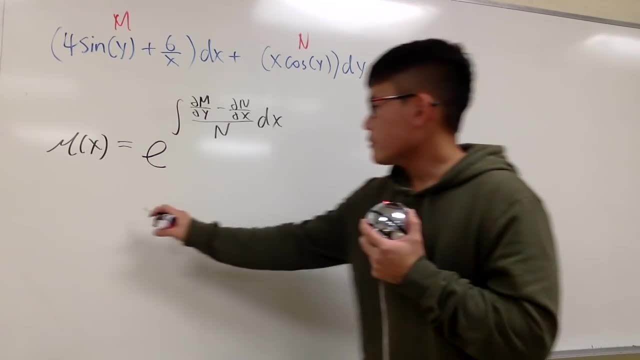 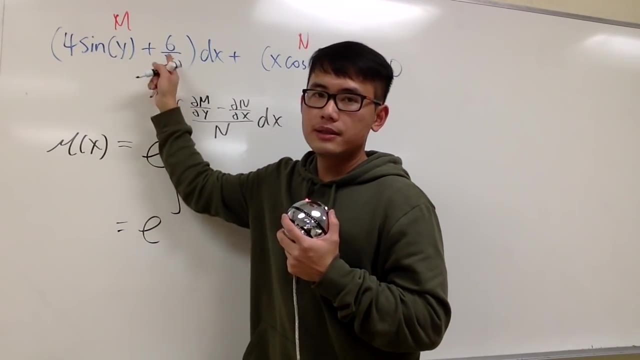 in terms of x only. Well, let's see, This is going to be e as the base. we have the integral as the power, partial m with respect to y. let's look at this. Well, we just have to differentiate this, right. 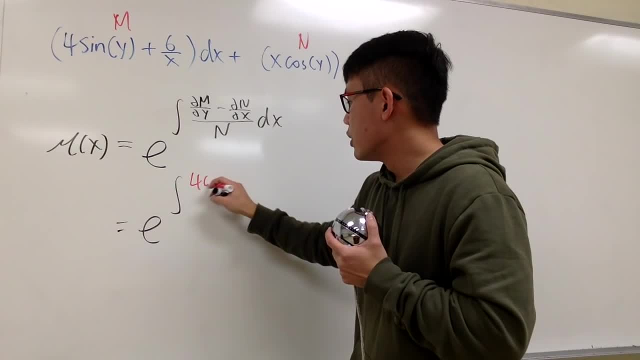 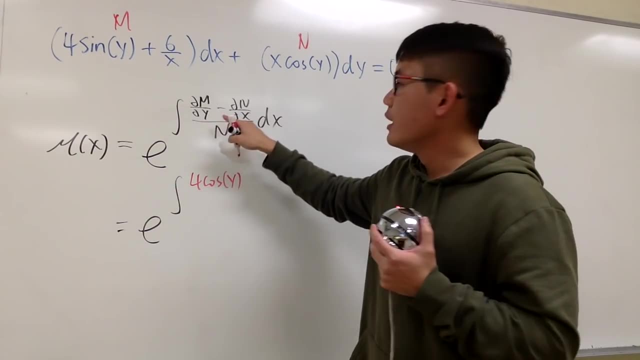 So the derivative of four sine y is going to be four cosine y, like this, And the derivative of this with respect to y is zero. So that's good. And now the minus. we have partial n with respect to x. Let's look at this and take the derivative. 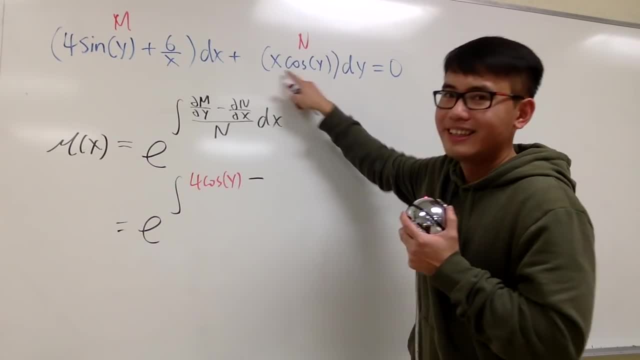 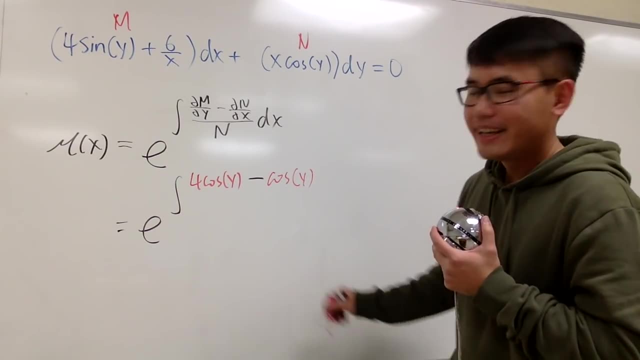 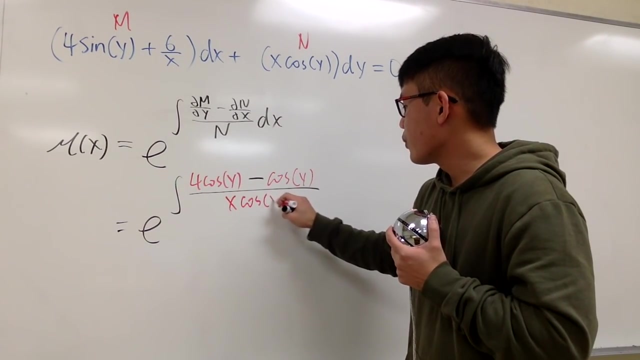 with respect to x, The derivative of x is just one and the constant cosine y it stays. so we have cosine y, right here, right. And then this is all over. n, which is that. So let's put this down as x, cosine y. 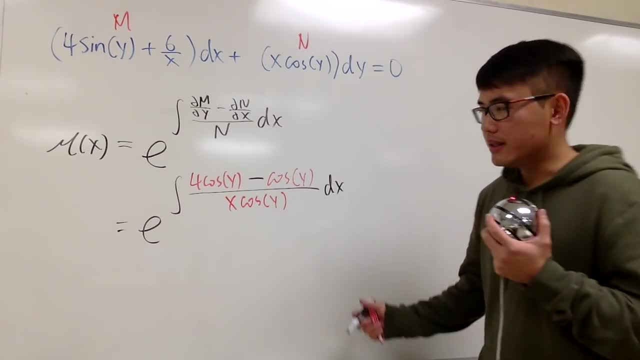 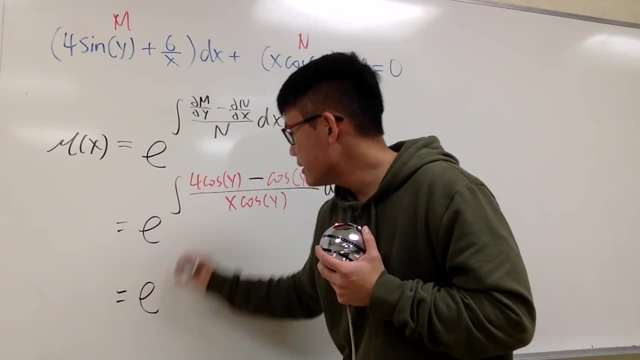 and we have the dx. Okay, let's see, We see y's, but hopefully somehow they cancel out Right here we have e as the base integral, four cosine y minus one cosine y, of course, that's three cosine y. 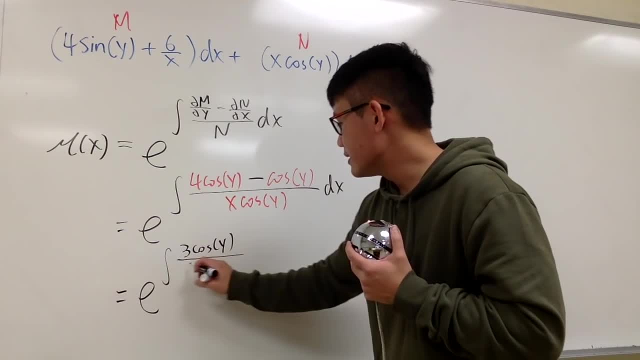 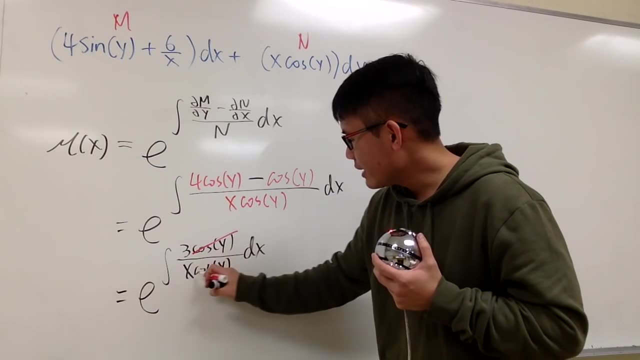 So put this down right here, Right here, over this is x, cosine y and we have this dx. And guess what? Look, cosine y, cosine y cancel each other out. So this right here is just going to be e. 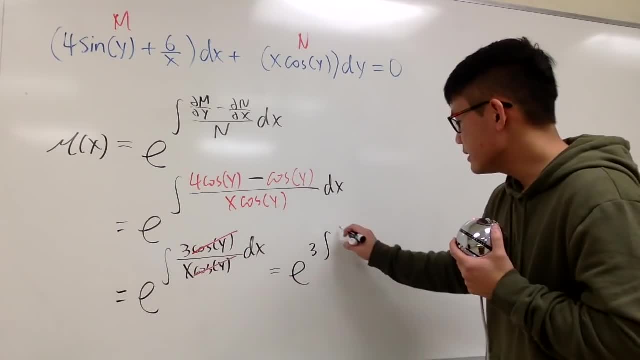 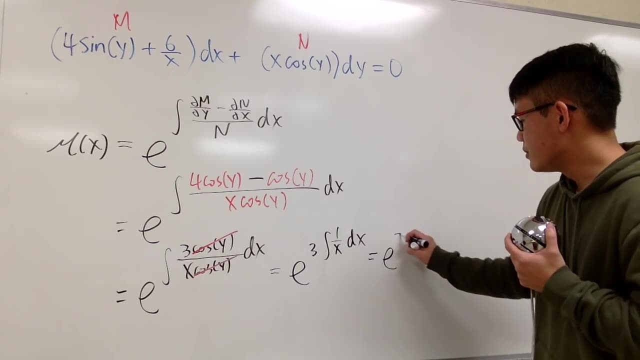 and that's bringing the three to the front. We have three, and then integral, one over x, dx, right. And now this is what? Well, this is just still e and the three is still three. Integral of one over x is just ln. 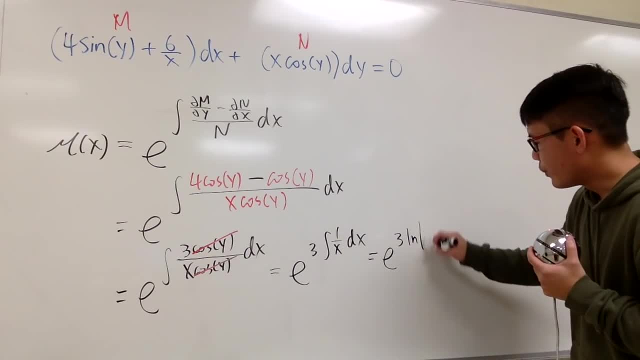 and you can put this down right And you can keep the absolute value for now, if you would like, I will for you, like this, But you don't need to put down a plus c, okay, And this is what we have. 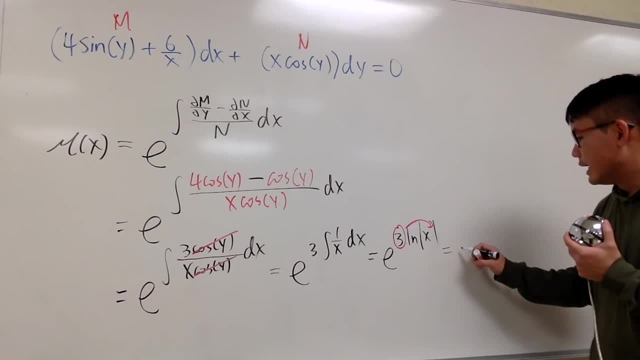 And of course you have to bring the three back here. So you have e to the ln absolute value of x to the third power, like this At the end: this and that will cancel And once again you can keep the absolute value for now. 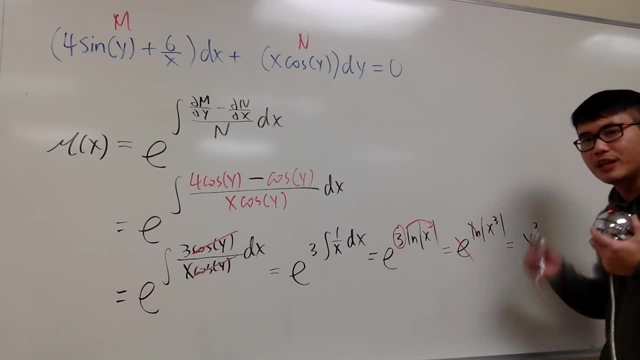 if you want, but you don't need to because, seriously, you just need to care about the function part. We have been talking about this many times already. So, seriously, you can just drop the absolute value, because this is what you need. 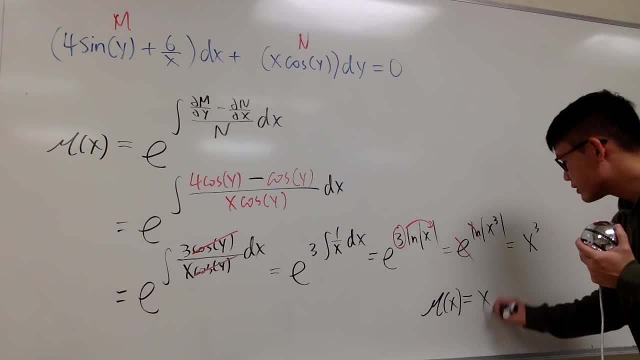 As you know, now, mu of x is x to the third power. This is all you need. okay, If you keep the absolute value, you have the choice between plus x to the third power or the negative x to the third power.